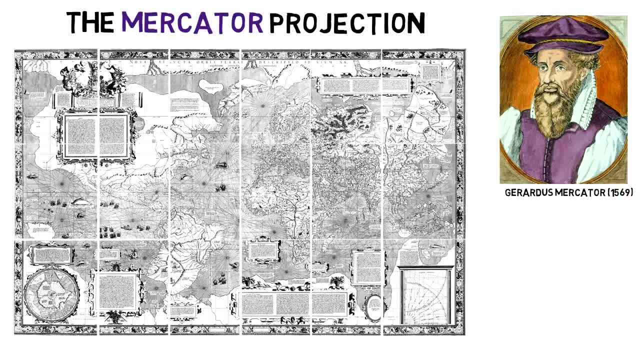 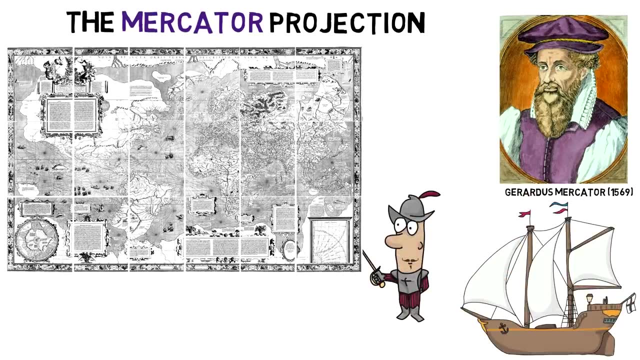 projection presented by Flemish geographer and cartographer Gerardus Mercator in 1569.. It's pretty old, and its generalized use has to do with the date in which it was invented. These were the times of the European colonialism and maritime discoveries, And so this map focused on 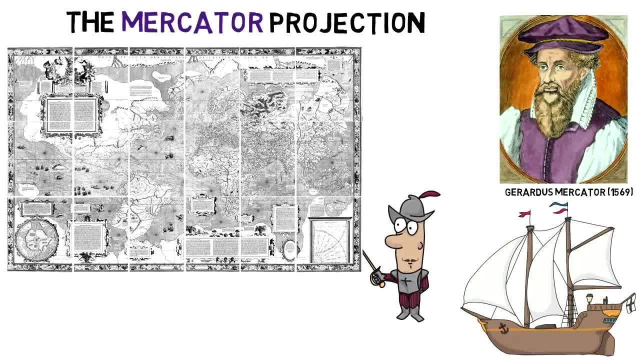 representing any constant course of constant bearing of a ship as a straight line, And so this map focused on representing any constant course of constant bearing of a ship as a straight segment on the map. To put it simply, if, in order to get from southern France to Canada, 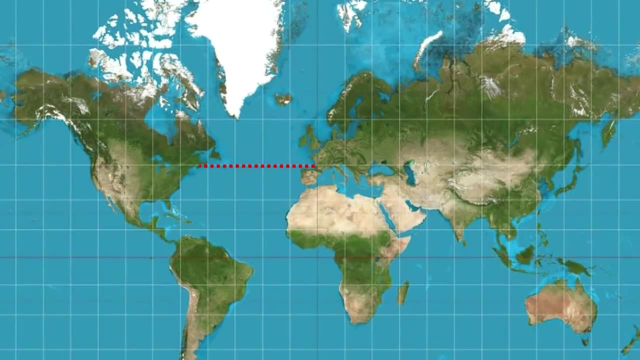 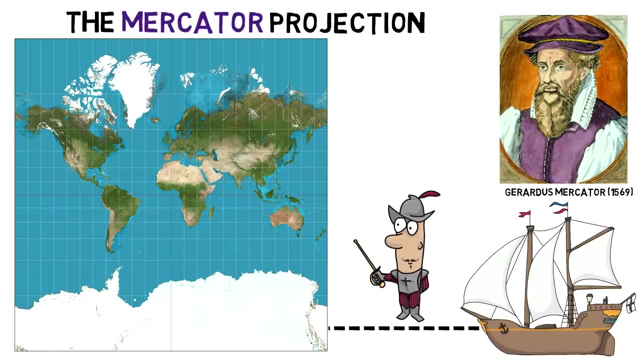 your ship had to just go forward and never turn, then the map would show a straight line between the two locations, And so this projection became the standard map for navigation. However, it has a big issue. The Mercator projection inflates the sizes of objects away from the equator. This 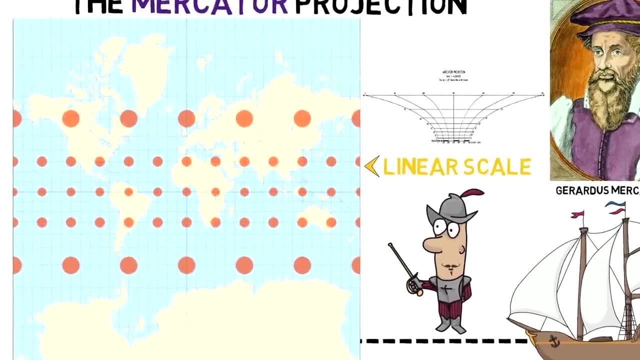 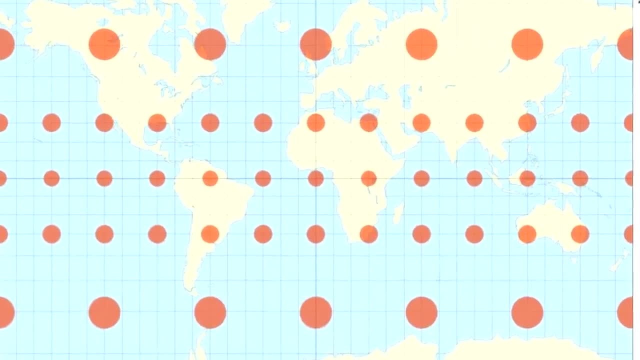 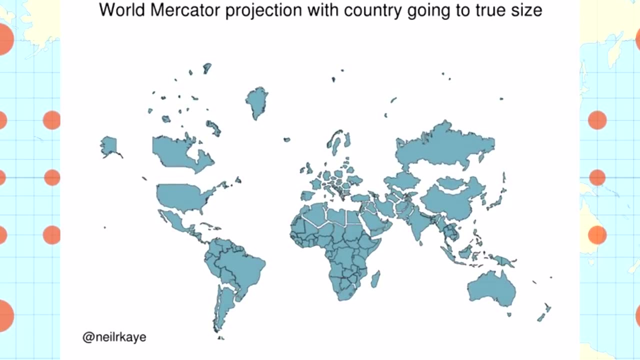 inflation is very small near the equator, allowing countries and continents there to be represented very accurately, but becomes distorted, being too big as it moves towards the poles. In this gif, we can see countries being reduced to their true size. The ones near the equator have little to no change, while the ones up north. 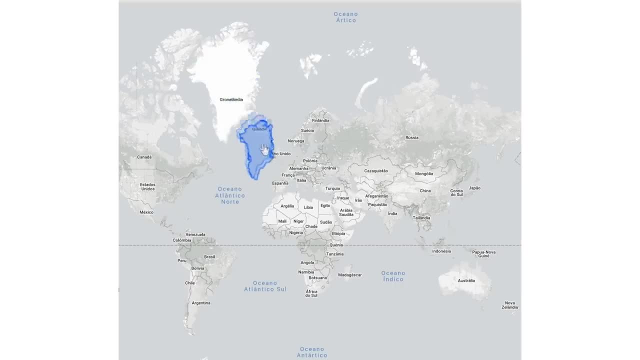 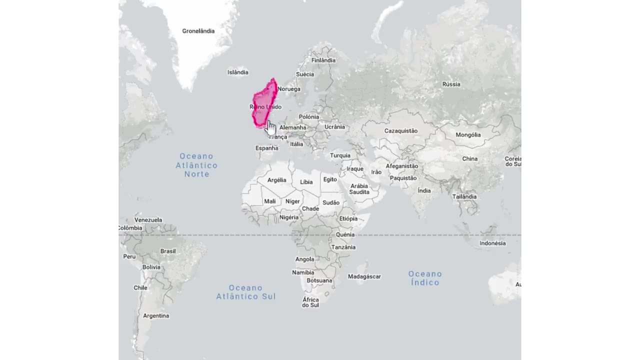 shrink a lot. Greenland appears to be the size of Africa, when in reality it is 14 times smaller. Madagascar looks the same size as the UK, when in fact it is twice its size. Alaska seems to be the same size as Brazil, when Brazil is 5 times bigger. 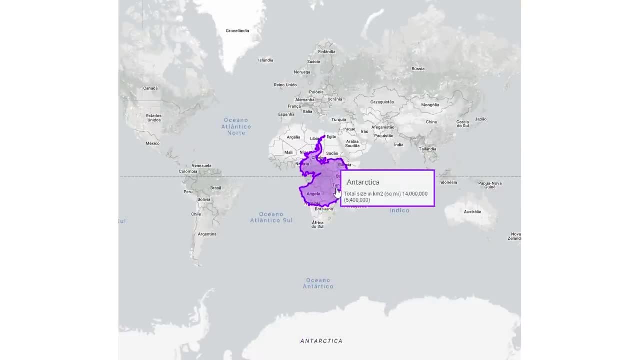 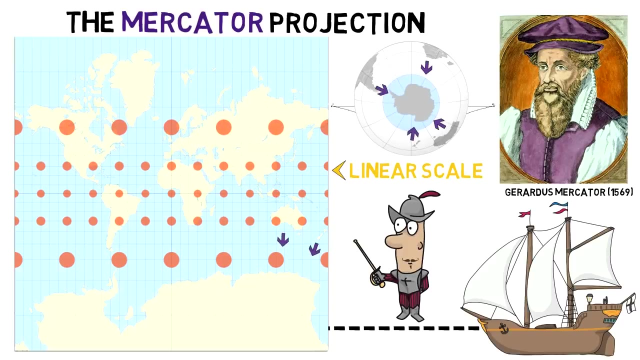 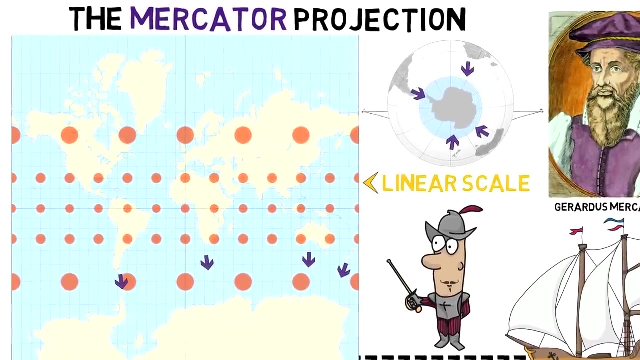 Antarctica looks gigantic when in reality it is reasonably small. It's just at the southern pole and so is reachable on a globe from all surrounding areas depicted here on the southern part of the map. And so, in order to depict that reachability, the map must show it distorted, like 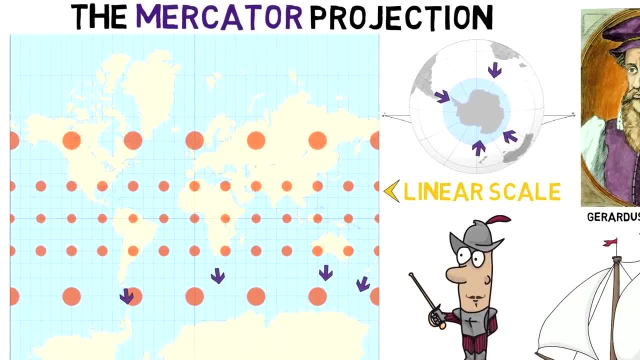 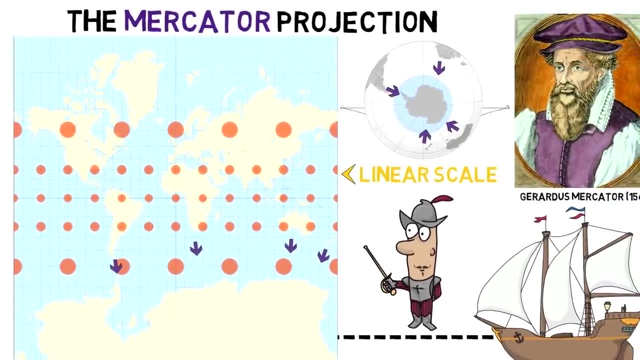 this. I made a video about this specific issue once regarding the true size of countries. Eventually, the Mercator projection has become a little less used- although I think it's still the majority of maps- But a lot of them switched to better ones which are more accurate. 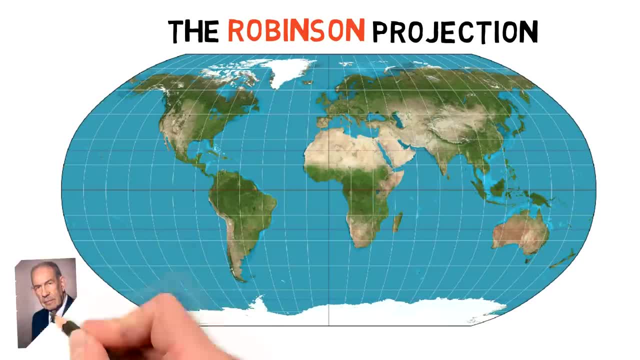 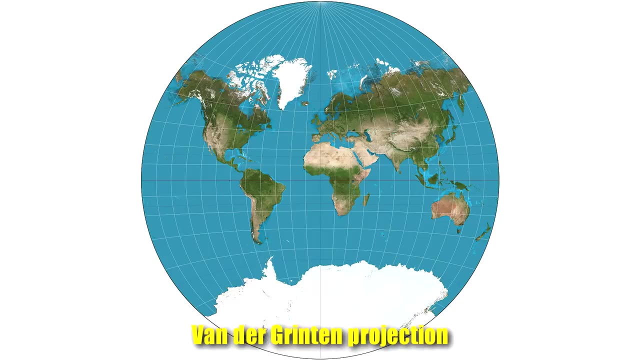 A good example, and one extremely used nowadays, is the Robinson projection, developed in 1987 and adopted by the US's National Geographic Society in 1988 as their official projection. Before that they used the Van der Grinten projection, which reduced Mercator's distortion in the center. 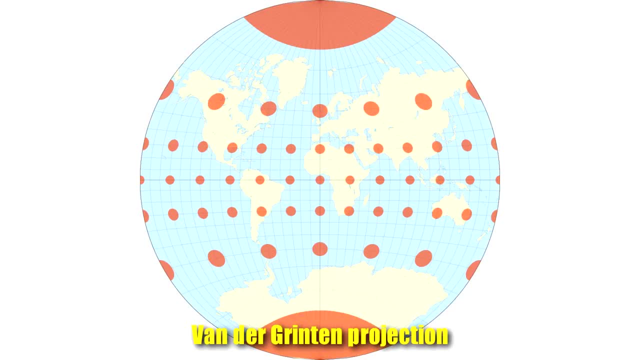 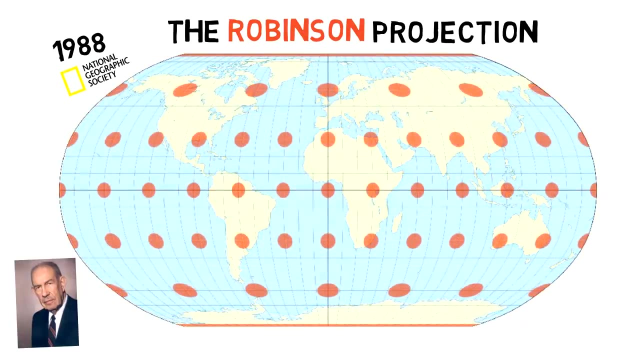 by concentrating all of it in the poles, which were extremely distorted, representing the globe as the center of the map. In this video, I'm going to show you how this projection works as a circle. The Robinson projection almost solves it entirely, though, and is honestly my 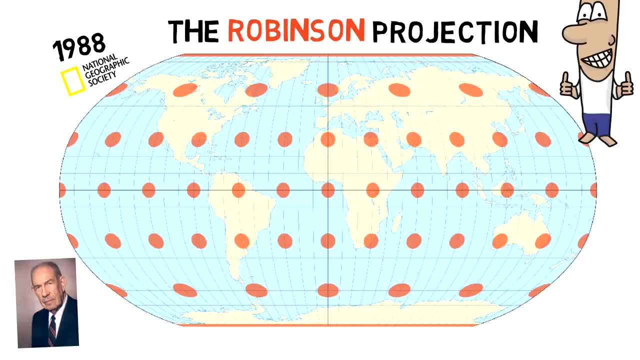 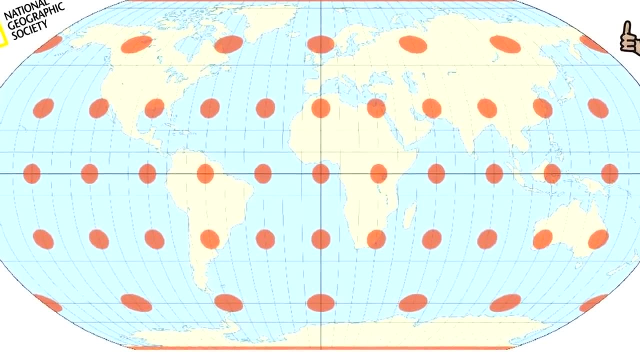 favorite one. because of this, The distortion in size is basically non-existent and only the actual poles are distorted, like we see with Antarctica, but something which I think is justified with the necessity of showing its accessibility from all areas of the south-southern. 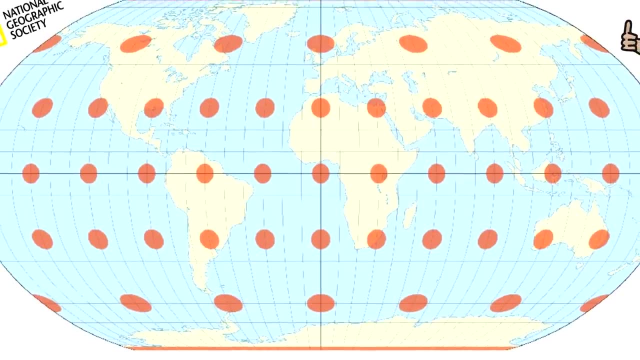 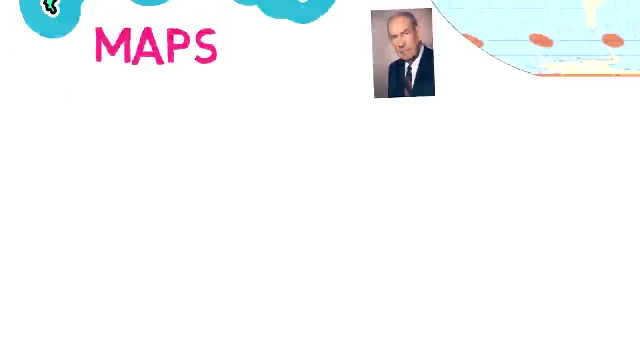 hemisphere. An interesting aspect in the majority of these projections is that the distortion is usually horizontally symmetric from the equator line. I'm sure there's some mathematical reason behind that. The Behrman projection from 1910,, for instance, shows a. 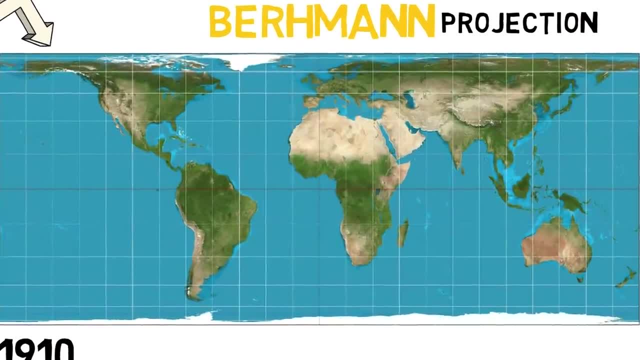 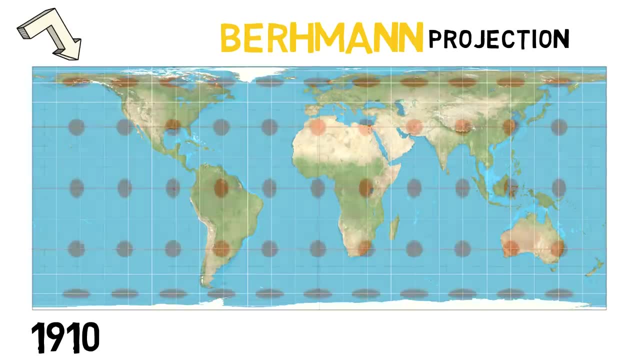 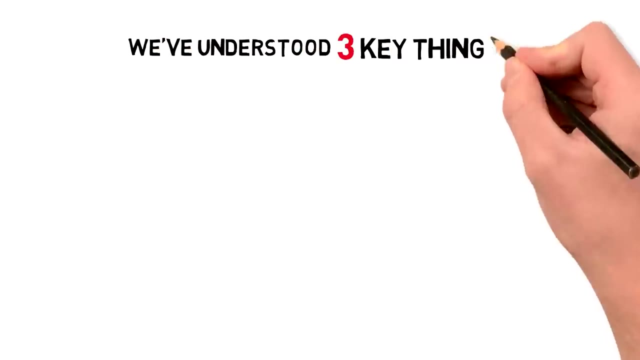 really weird looking: Central America, South America and Africa. They are way too disproportionately big when compared to North America, Europe and most of Asia, But they are disproportionate in a symmetrical way. So now we've understood three things. One: all maps are distorted because it's 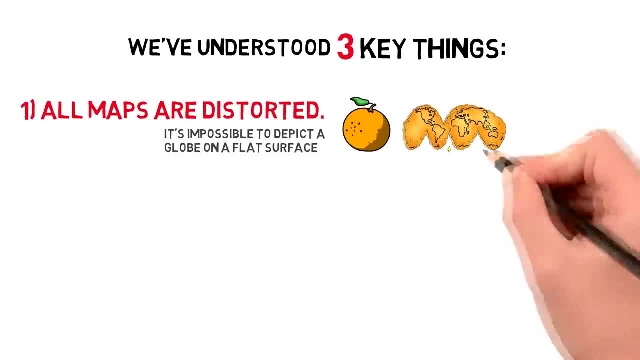 impossible to depict a globe on a flat surface. Two: the type of distortion the map has depends on what it is, What it was made for. The Mercator projection was made for ship traveling, and so it prioritizes that. The courses and directions, Sacrificing object proportions in some parts of the map. And three: 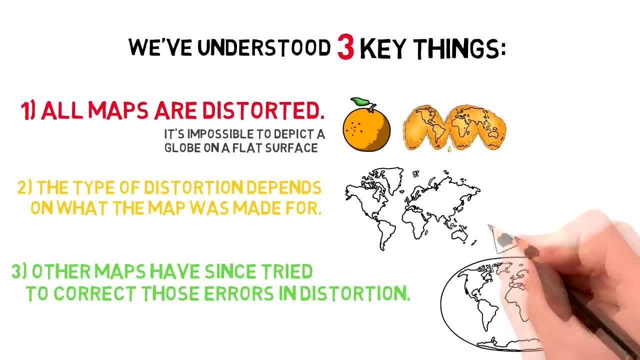 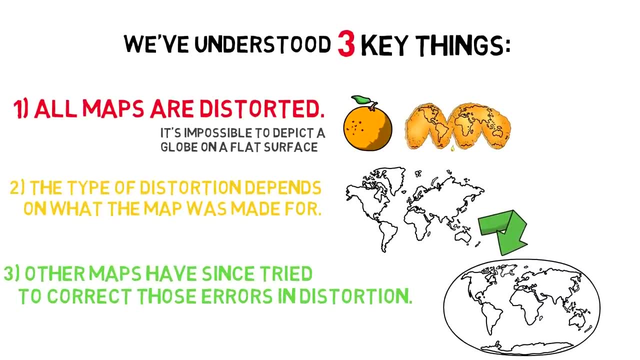 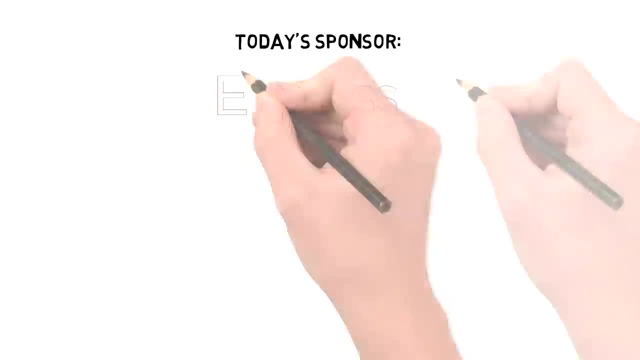 other maps have since tried to correct those errors in distortion, Either prioritizing other aspects or attempting to depict our continents in the most accurate way possible on a flat surface. This is why there are so many projections. Before we go on with the video, a quick message about 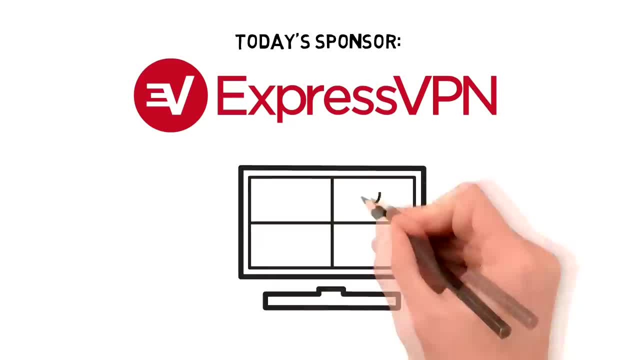 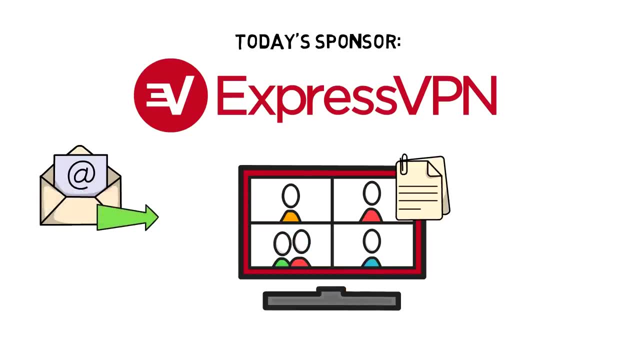 today's sponsor, ExpressVPN. Whenever we are online, we're divulging information. Either we are aware of it by, for instance, sending someone a message, or we're not, And websites we visit retrieve it from us without us knowing. they do Like information about you- your IP address. 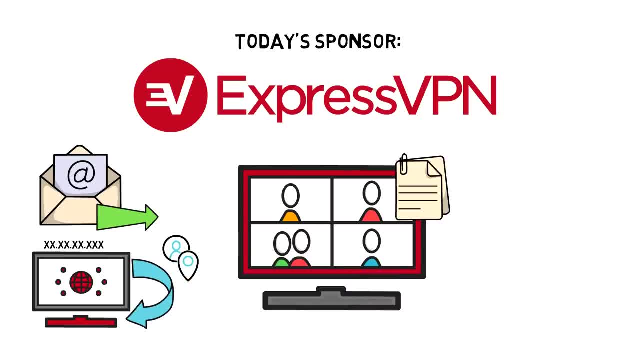 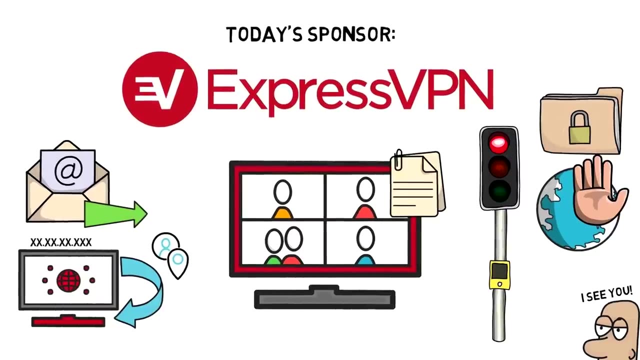 or location. Plus, your internet service provider knows everything you do as well. ExpressVPN puts a stop to all of that by encrypting your data and hiding your location. This way, hackers, websites and service providers can't access your data and use it for negative. 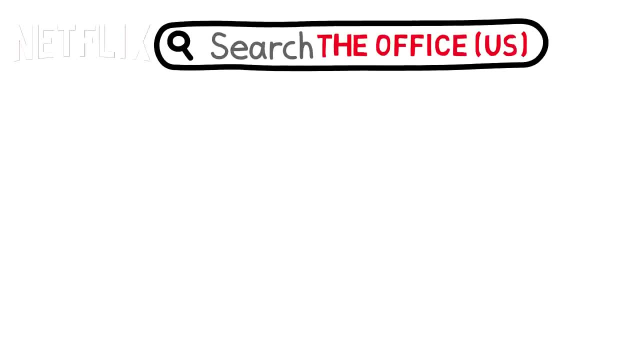 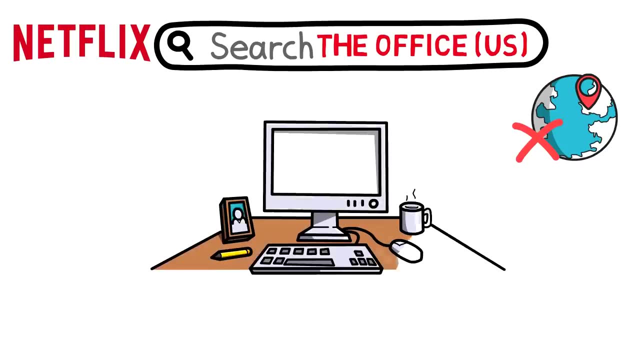 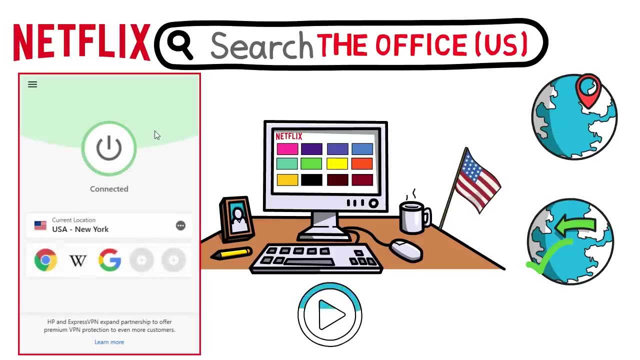 things. Plus, you also get the added benefit of being able to visit websites that are geo-restricted. I recently wanted to watch The Office on Netflix, but that isn't available where I live, and using ExpressVPN allowed me to switch my region to the US, accessing their catalog. 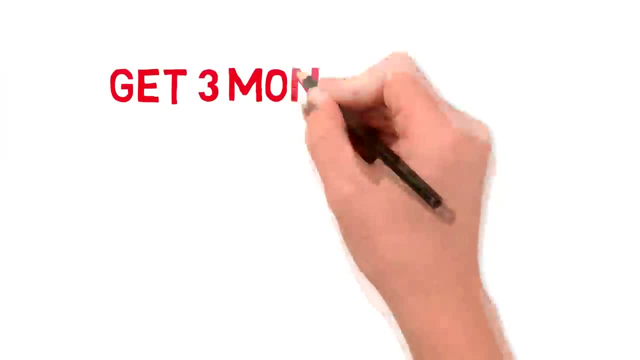 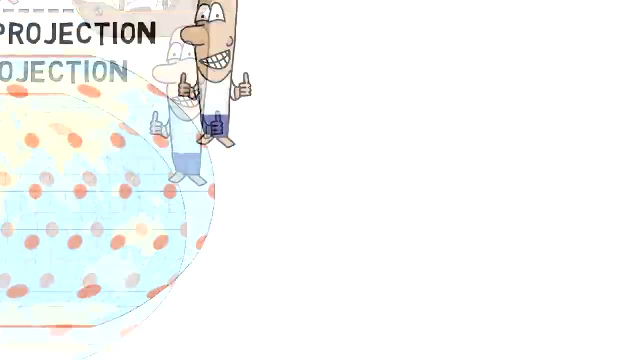 and watching the show. Find out how you can get 3 months free by clicking the link in the description below. Thanks for watching and I'll see you in the next video. All these maps we've seen so far have been, however, pretty standard and straightforward. 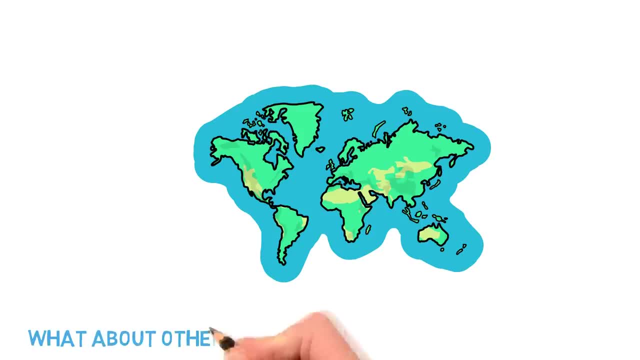 in the sense that they are the way we expect a map to look like. But what about all the other projections that look way different? Let's start with this one. This is the transverse Mercator. Essentially, it stems from the Mercator projection, but depicts it in a different shape. 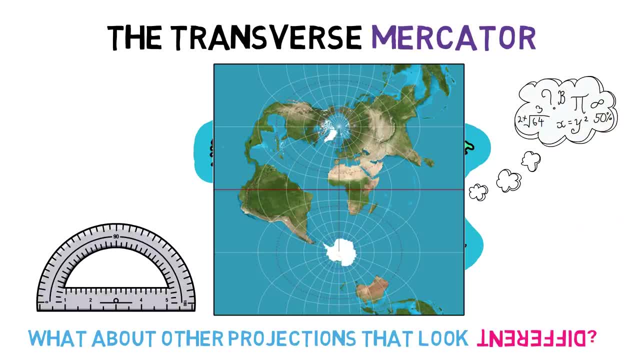 slash angle. Now again, I'm totally ignorant regarding the math behind this, but it's in the math that the difference is, And that's something out of my area of expertise. But there is the obvious difference in the visual aspect. Here the pole's sizes are pretty much near. 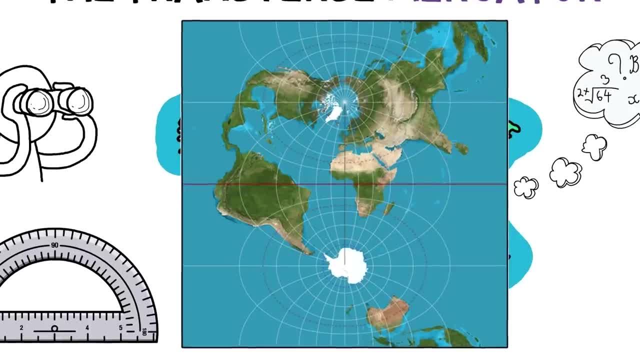 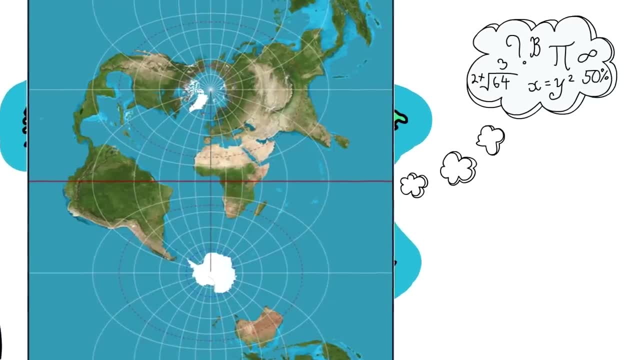 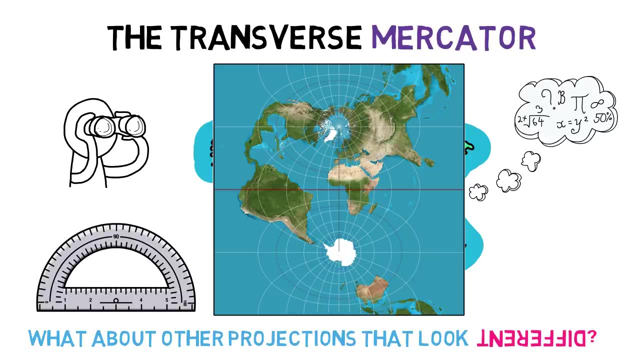 perfection, but other areas suffer as a consequence. Southeast Asia is way too big, as is South America, but Antarctica is perfectly depicted. So if we were to use the two Mercator projections side by side, we would have an almost perfect depiction of our world. We also have 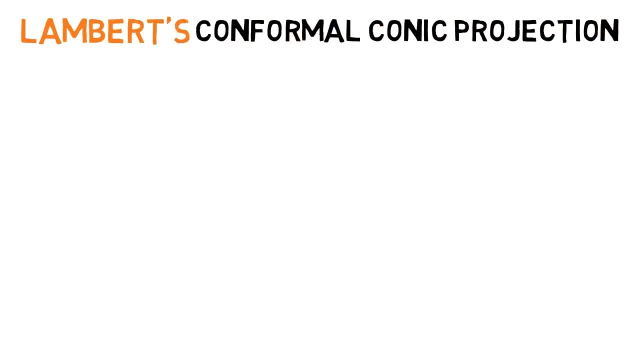 examples of maps which are very similar to the ones we've seen so far, but with a different shape, Which didn't have to deal with Antarctica's problem because, well, when they were made, Antarctica hadn't been discovered yet. Lambert's conformal conic projection from 1772 is a good 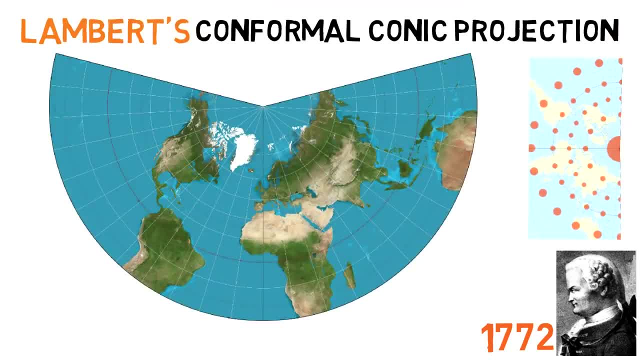 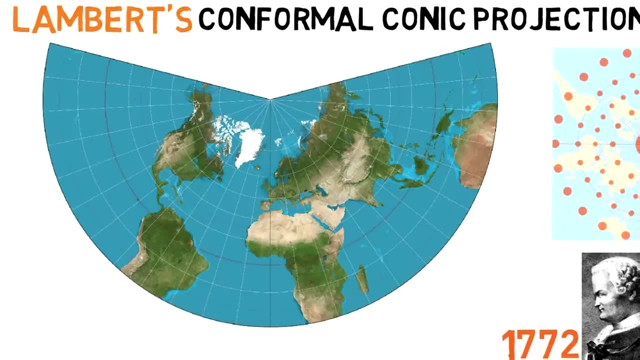 example of this, And it's actually extremely proportionate in pretty much every aspect, Although it is missing the tips of South America, South Africa, Australia and New Zealand entirely. This map projection is apparently still the basis for a lot of the aeronautical charts used by air. 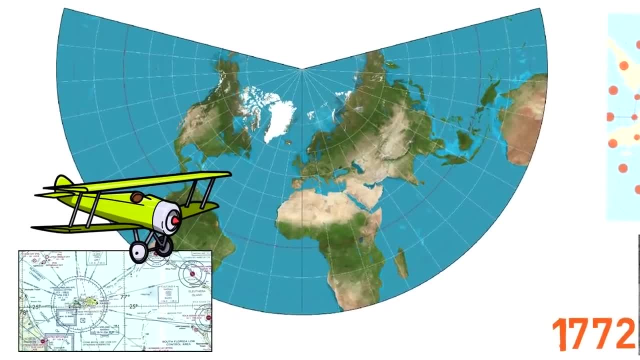 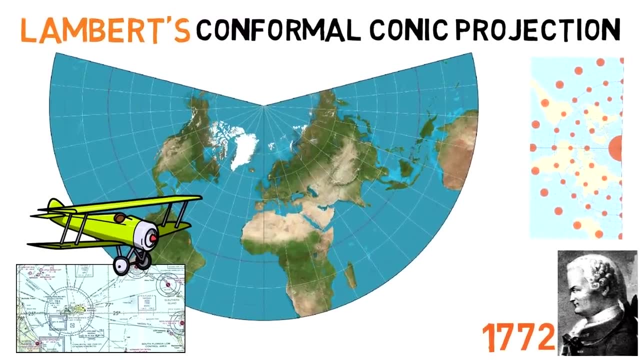 traffic controllers. So if we were to take a look at the map projections, we would see that the map projections are actually very similar to the ones we've seen so far, but with a different shape. What we therefore understand is that, essentially, when cartographers and geographers 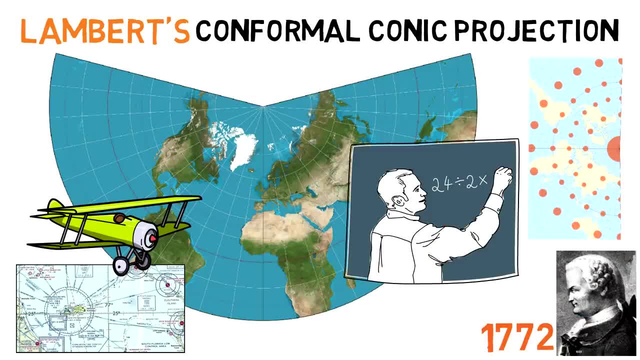 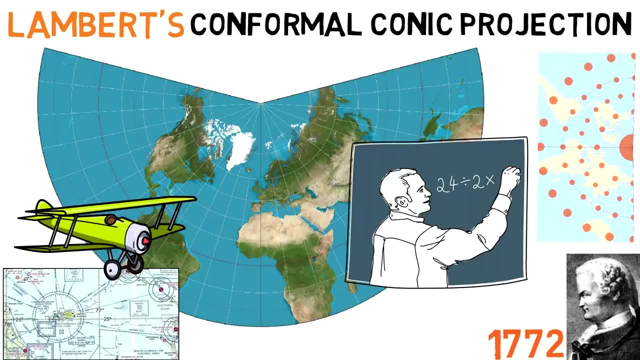 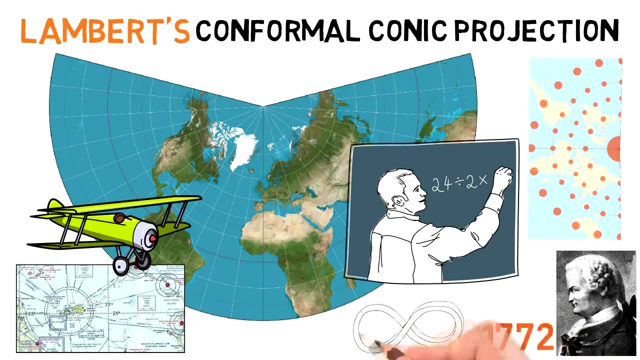 develop these map projections, they always come up with specific mathematical principles behind them, And these principles can still be used today, even if the original map projection itself is not because it became outdated. That's why the amount of map projections is virtually infinite, because we can always change something in a projection's equation. 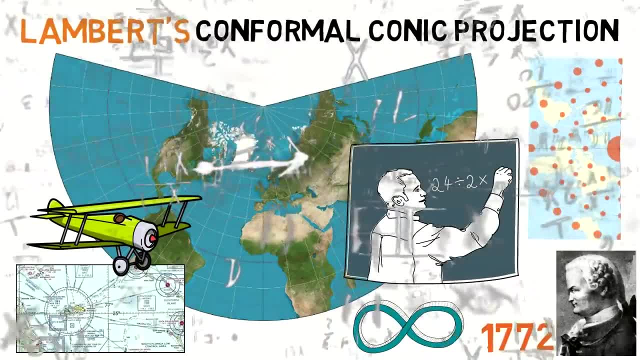 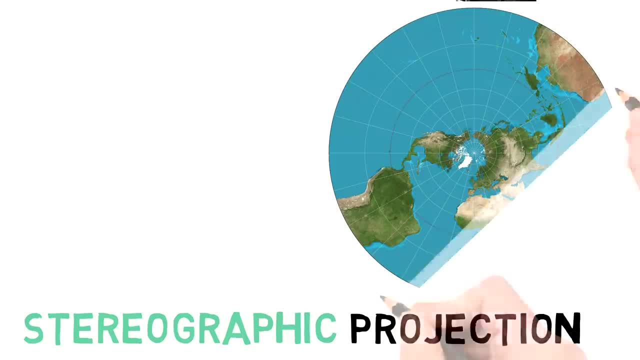 even if a tiny detail, or come up with an entirely new projection. Another example of a perhaps outdated projection is the stereographic projection. All of these have really complicated and technical names that I don't understand either, so the best way to understand them is by seeing how they look. 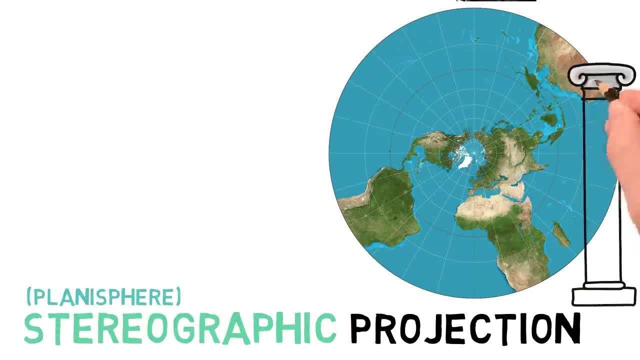 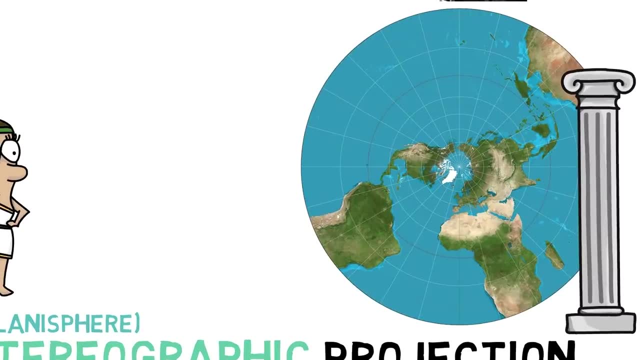 This one is also known as a planisphere projection, and it dates back to antiquity, having been used in some of ancient Greece and Rome's maps Depicted on a circle. instead of being centered on the equator, it is centered on the north pole. 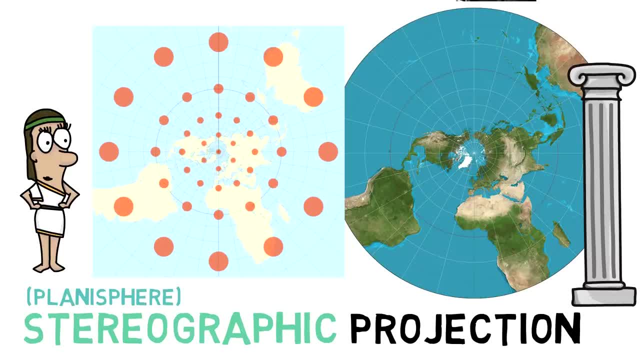 with an increased level of distortion as you move away from it. But the errors were excusable because the point was to depict the northern hemisphere with a high level of accuracy. However, some more recent projections just wanted to depict all continents with the minimal error possible. An example of that is the Airy minimum error projection. 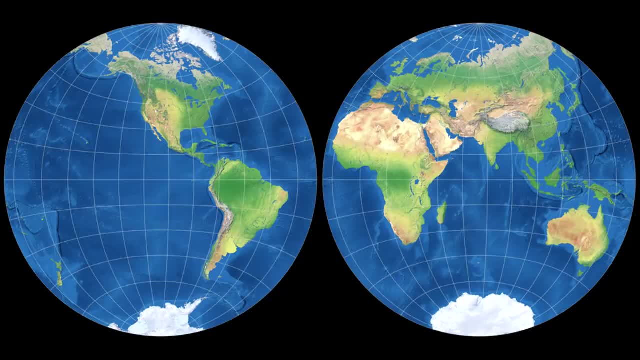 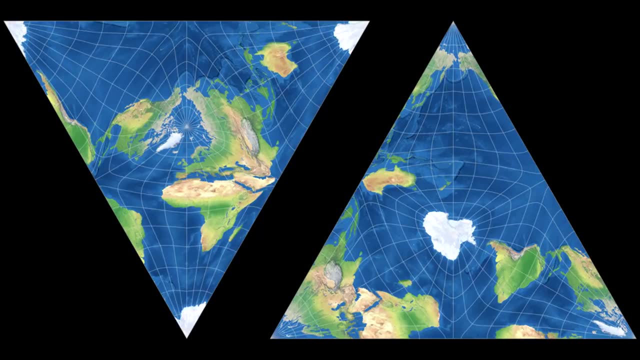 which pretty much took the globe, cut it in half and put two circles side by side. Some follow the same trend and use two different surfaces put together, like Van Leeuwen's GC, which uses two triangles, or Adam's hemispheres, which uses two Lozangs. 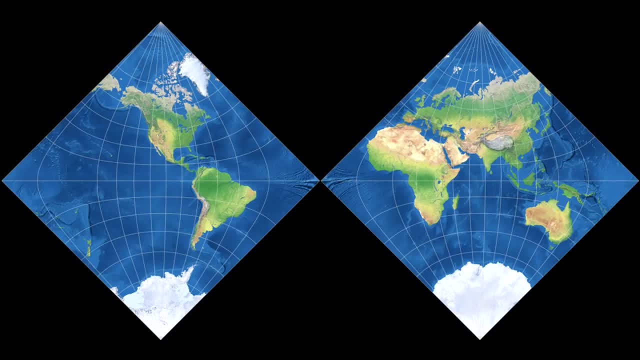 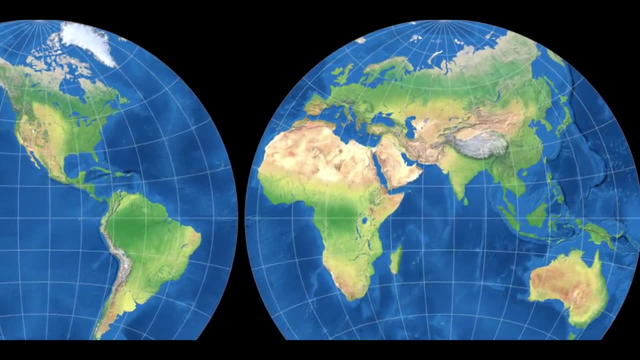 This circle one is very accurate, but still not perfect, because it's not possible to demonstrate the curvature of the globe in the central part of the circle, And so these areas here- Russia, the Central Asia, Istan or India- are a little too far stretched when compared with Italy or Ireland. But it's not a problem because the curvature of the globe is not the same as the curvature of the globe in the central part of the circle, And so these areas here- Russia, the Central Asia, Istan or India- are a little too far stretched when compared with Italy or Ireland. But it's not a problem because the curvature of the globe is not the same as the curvature of the globe in the central part of the circle, And so these areas here- Russia, the Central Asia, Istan or India- are a little too far stretched when compared with Italy or Ireland. 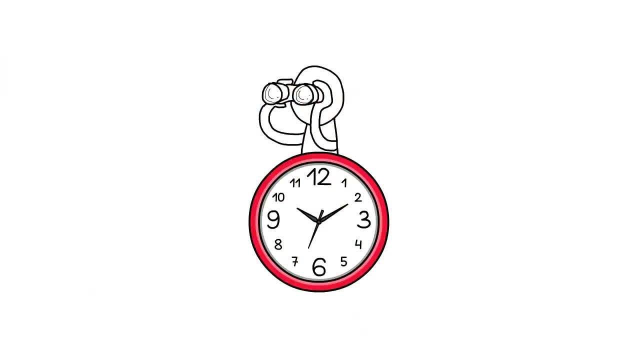 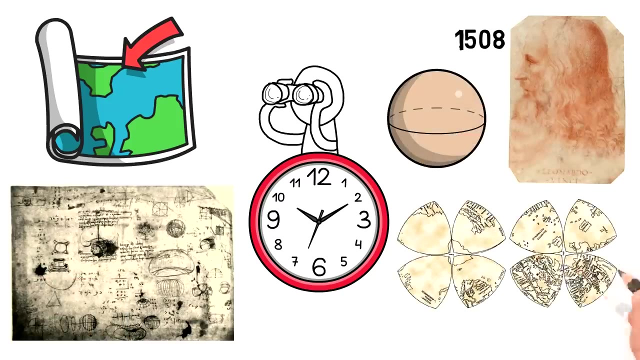 We could stay here for hours just looking at map projections, but I think at this point we've understood the basic principles behind them and why they are so different and vary so much. Like a projection proposed by Leonardo da Vinci in 1508, which set the path for Cahill's butterfly projection. 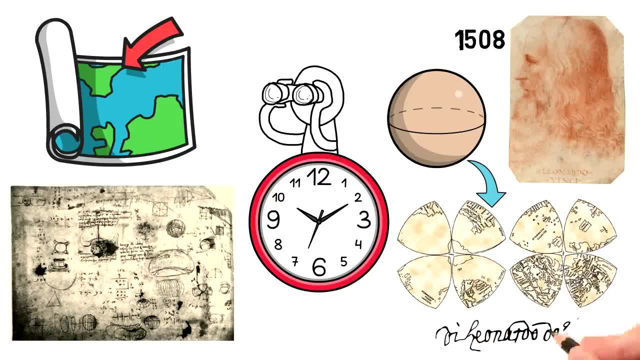 by attempting to divide the globe into eight pieces. So I'm just going to show you two or three more that I found really cool looking and that are amongst the most unique out of the currently existing models. First, the one I just mentioned, which comes from Leonardo da Vinci's ideas, the Cahill Conformal. 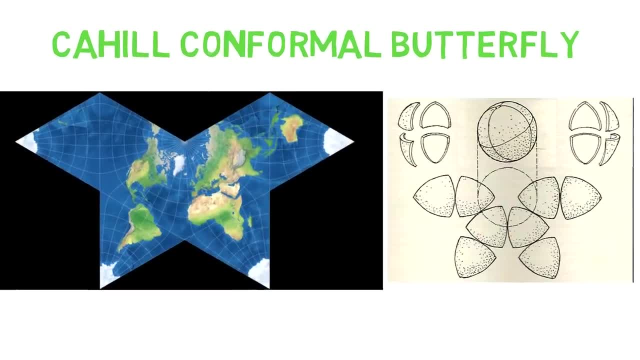 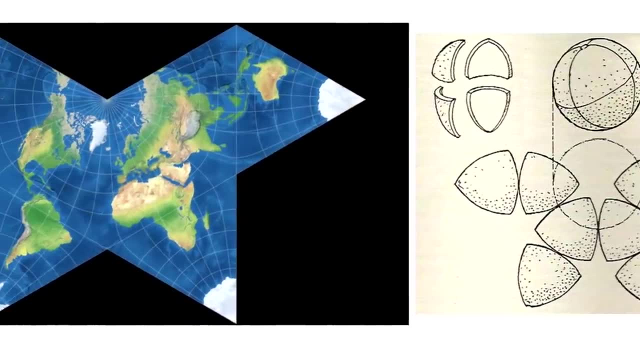 Butterfly. In it we see the world depicted in eight triangles And honestly it might not be in the orientation we're used to, or in a rectangular depiction, but I kind of love it. Look at the accurateness of the sizes, the precise depiction of Antarctica's reachability. 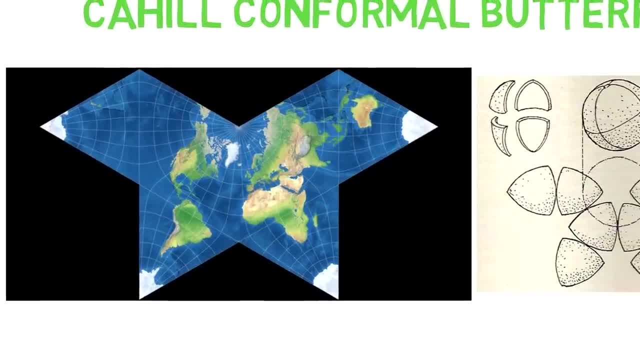 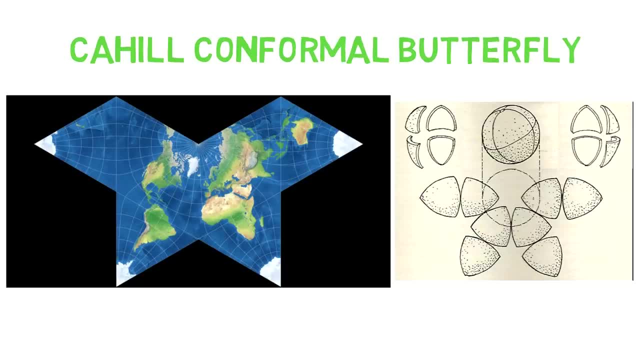 without having to stretch it to no end. It's just totally brilliant. Plus, the issue we have of certain continents being split can be solved by moving the world. So let's take a look at the Cahill Conformal Butterfly in the triangles. according to our desire, These are visible in: 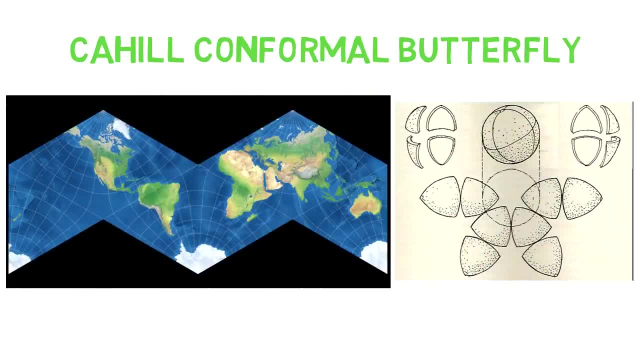 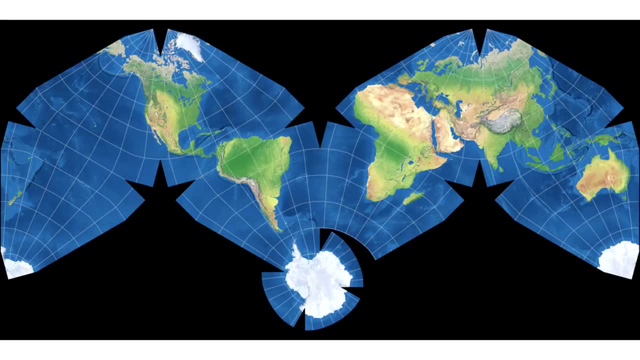 other forms of arranging this projection, like the Cahill Conformal M-shaped. There's also the Cahill Keys projection, which depicts the world also in eight triangular shapes, although one of them has an additional piece for Antarctica. There is also a cool one called the Chaiselange Conformal, The. 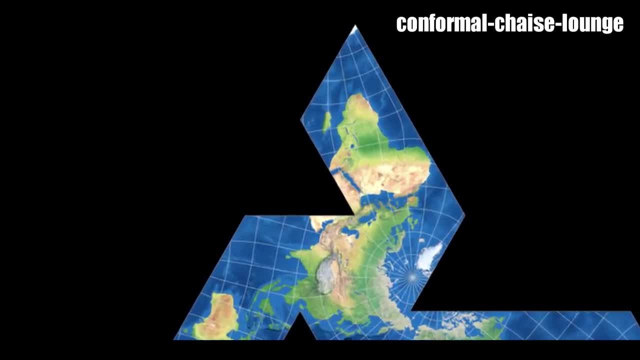 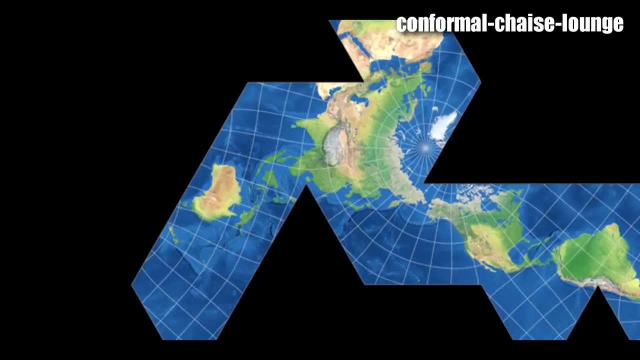 name, I guess, comes from the fact that it looks like one. It's pretty good and despite not looking like it because it's separated, it shows us the entire world very accurately. So let's take a look Very accurately. However, I feel the way of dividing it isn't the best because it takes 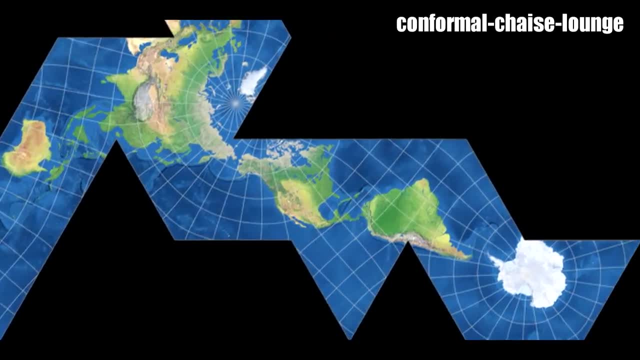 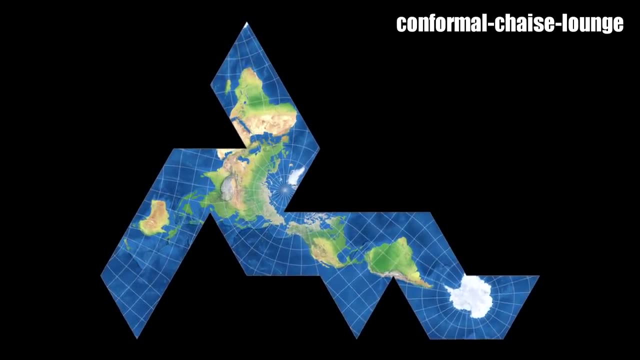 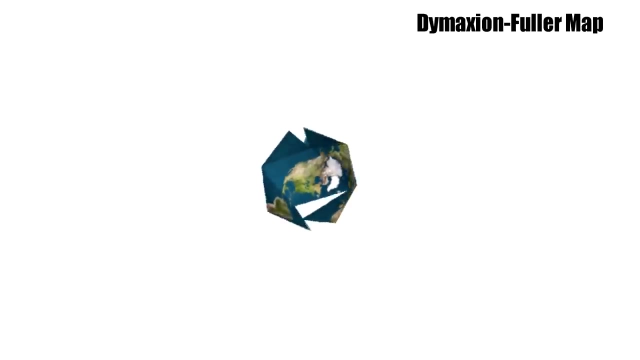 away our notion of distance, and if we didn't have pre-existing knowledge of where things are in relation to each other, it would be kind of useless in terms of serving its purpose as a map. Then the De Maxion-like Conformal from 1943, which attempts to transform the sphere into an 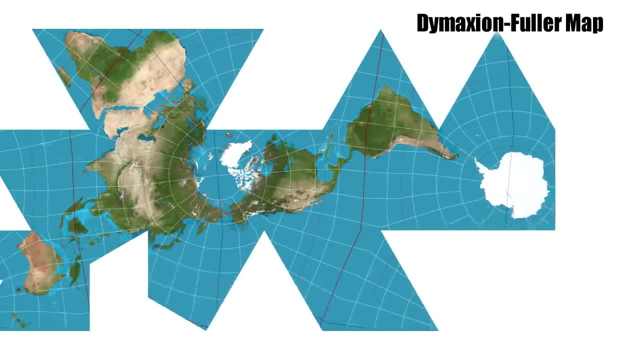 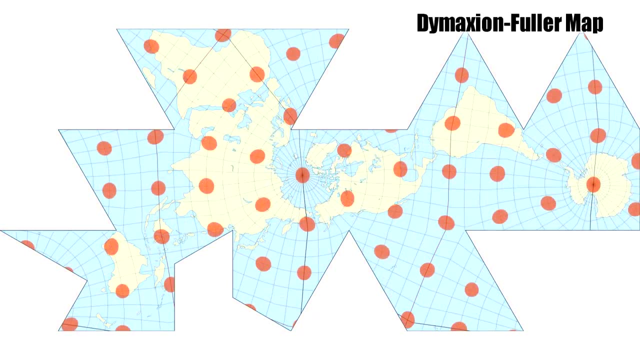 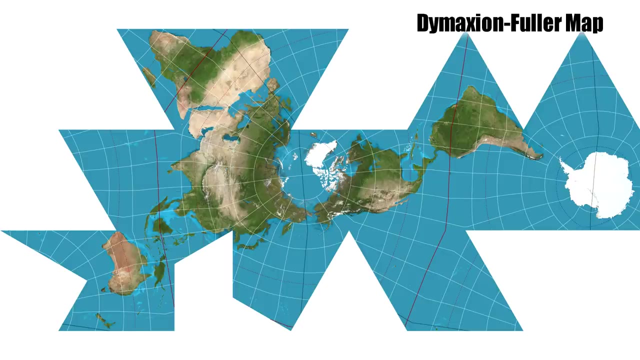 icosahedron, a shape with 20 sides, then flattening out those 20 sides on a surface. It preserves shapes and sizes very well, but is heavily interrupted as a consequence. But to be fair, I think at this point the goal of the makers wasn't to create a useful map in the sense of 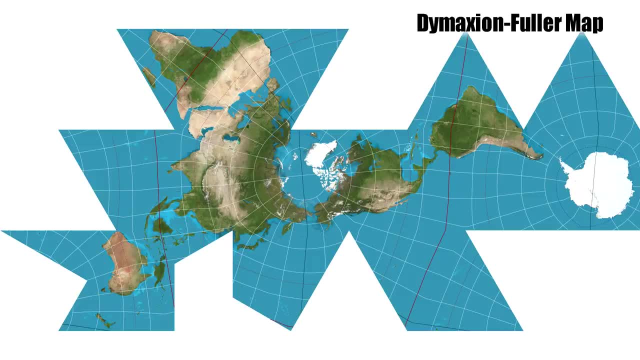 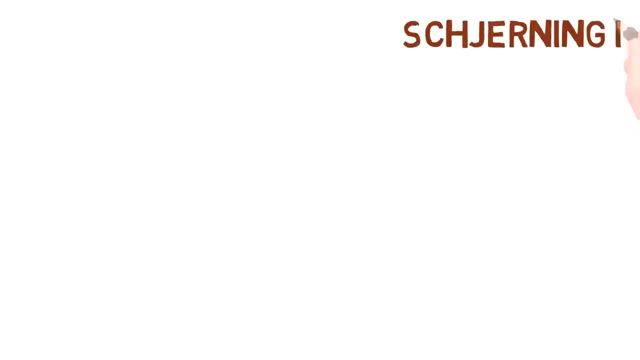 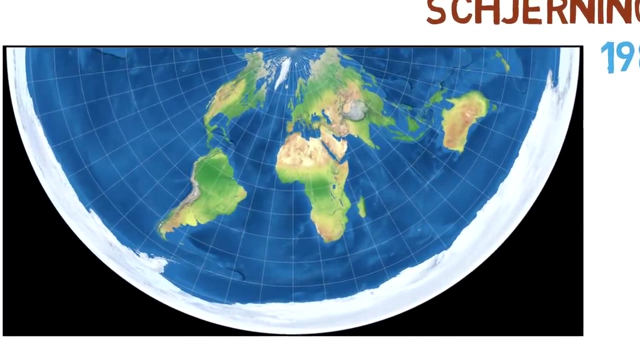 it being good for navigating via sea, land or air. They were or are just trying to make the most accurate depiction of a globe on a flat surface. And finally, the Schierning 1 from 1982, which I just find extraordinary because it really takes the whole stretched Antarctica.